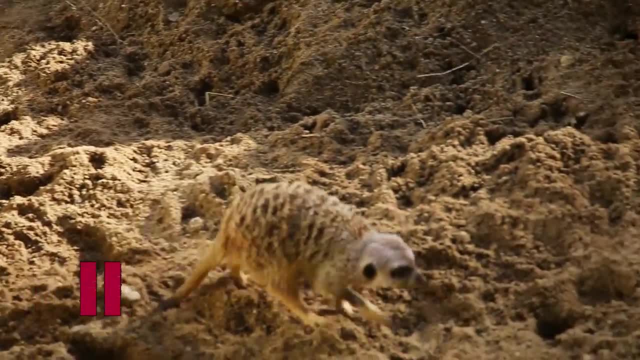 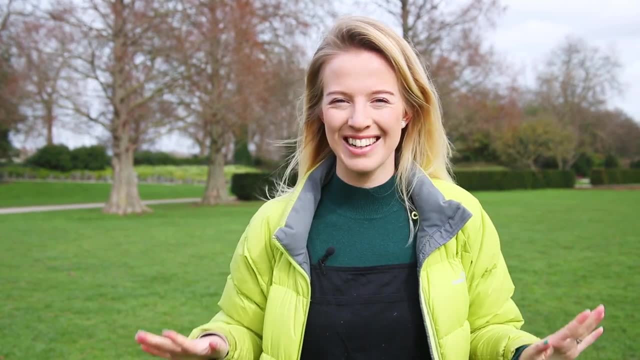 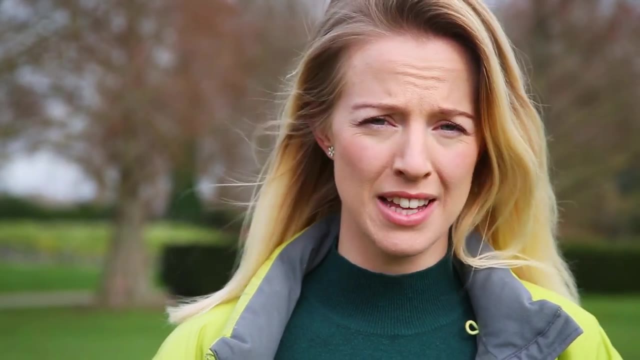 go and I'll see you back here soon. Good you're back. I hope you're feeling better and the school is feeling better And much cleaner. now Let's take a look at the earth's resources. Some of them are renewable and they can reproduce themselves like plants and animals. But in saying that, we need to 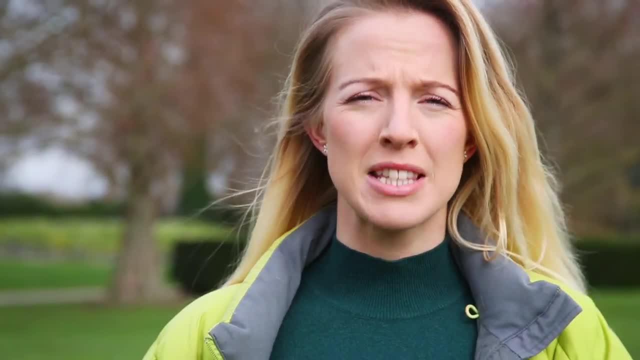 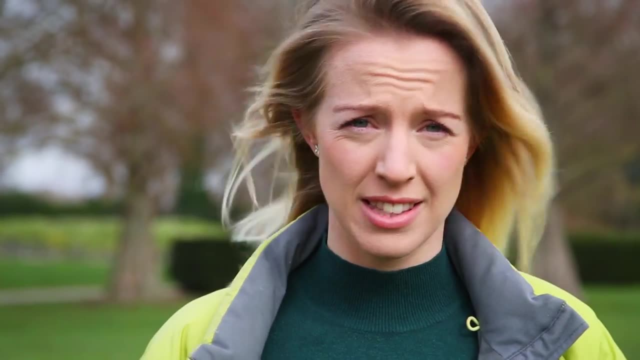 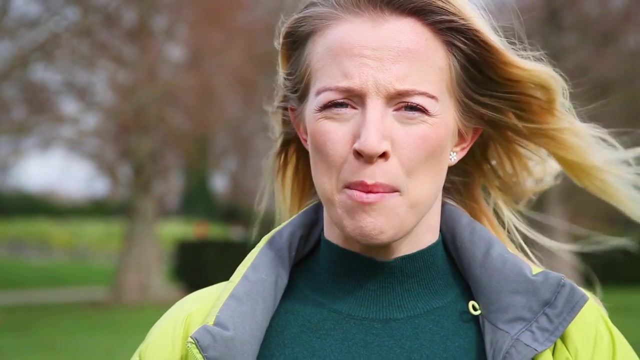 make sure we're always taking care of them as well. But some of the resources are not renewable, meaning that when they're gone, they're gone for good. That's it. Fossil fuels like petrol and oil are used for cars and many other things, But the more that is used 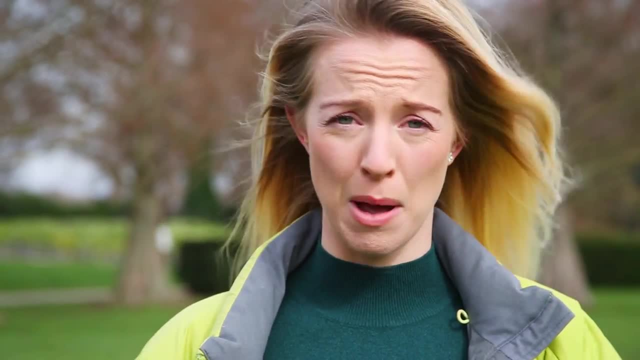 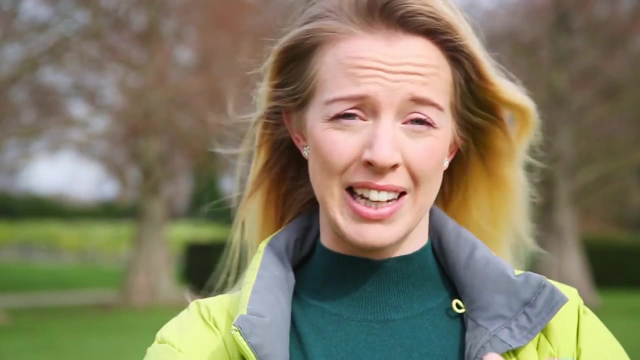 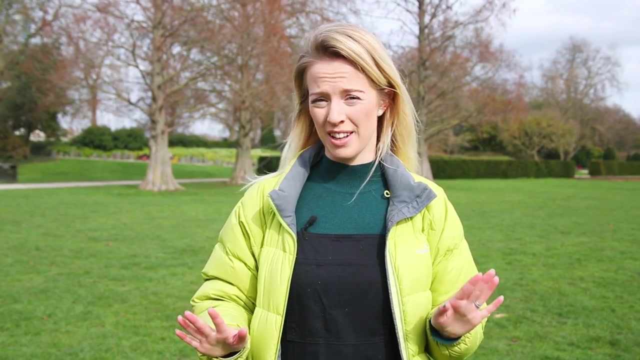 and burnt up, the more that they're going to have to take from our beautiful earth. Luckily, there are a lot more options nowadays for how you can run cars like electric cars and hydrogen cars. I wonder what they'll think of next. 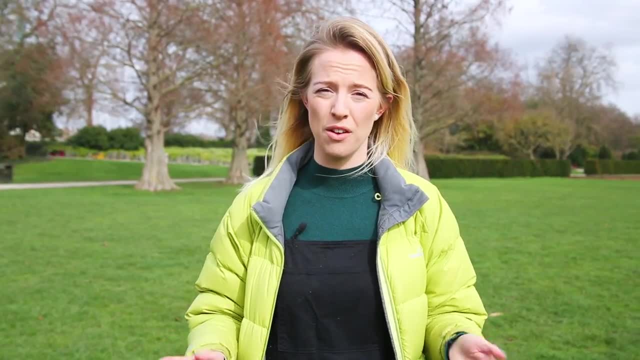 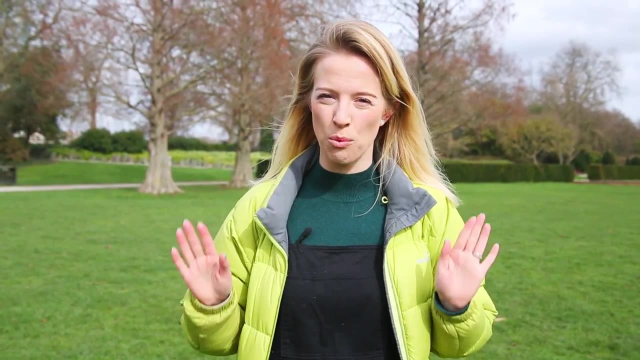 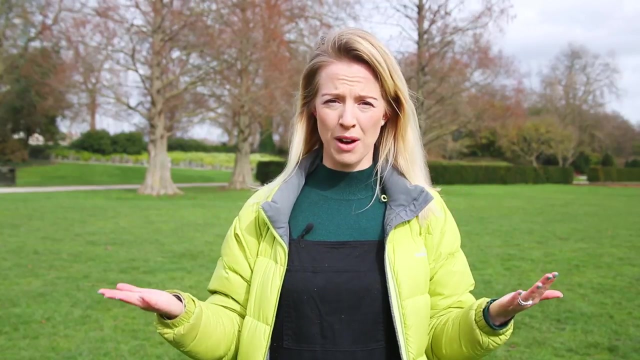 Water is another one of the earth's resources that we need to be careful of and conserve. With the amount of people on this planet, we need to make sure that no one is wasting any water. There may be times of drought, meaning that there is no rain falling. If there's no rain, 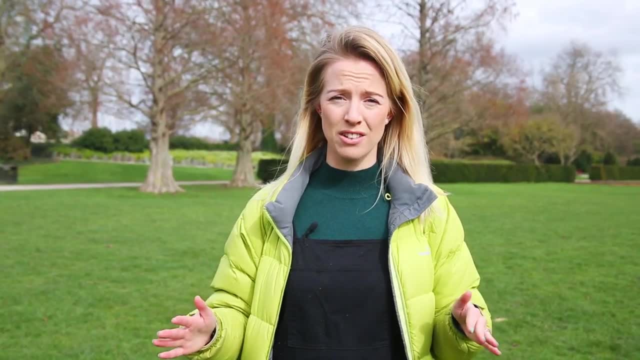 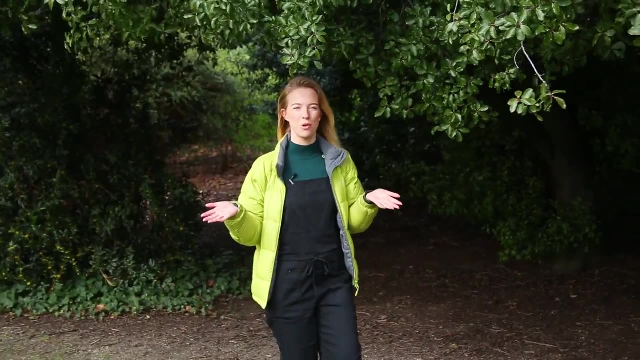 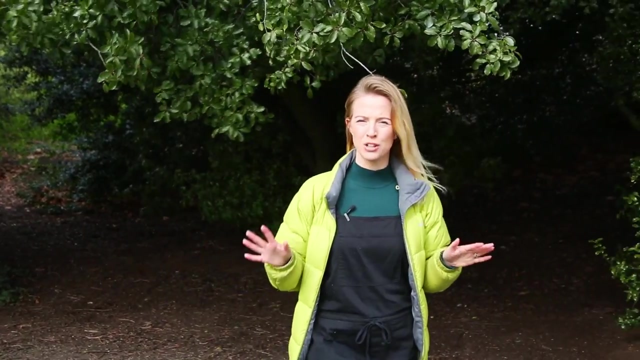 falling, then the water dries out. If the water dries out in certain areas, that might mean that food crops will die out. Now that we know a little bit more about the earth's environment, let's have a talk about some of the habitats of the animals in the world. People are using everyday items that 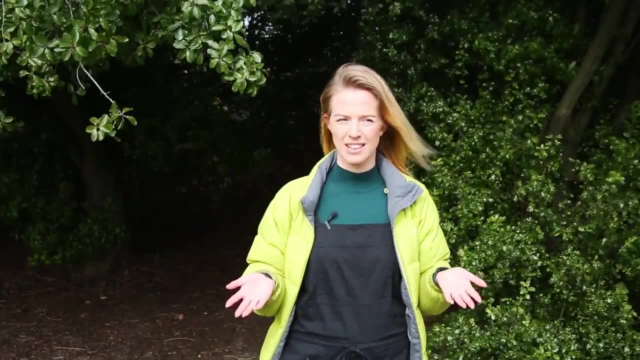 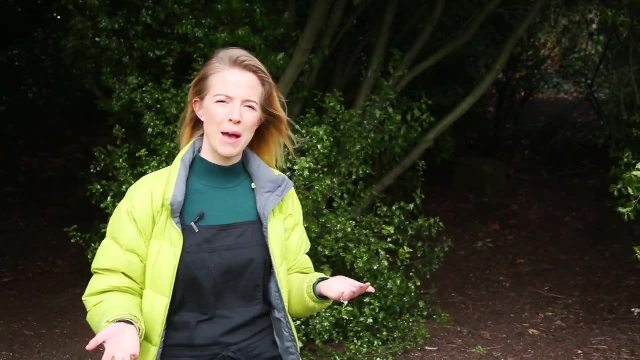 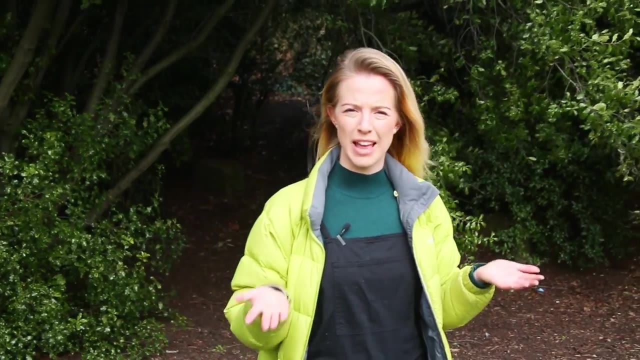 they may not realise are harming some of these habitats. Let's take Paper, for instance. Paper is made from trees. The more paper that people need to use, the more trees will be cut down. But think about the animals that live in the habitats of the 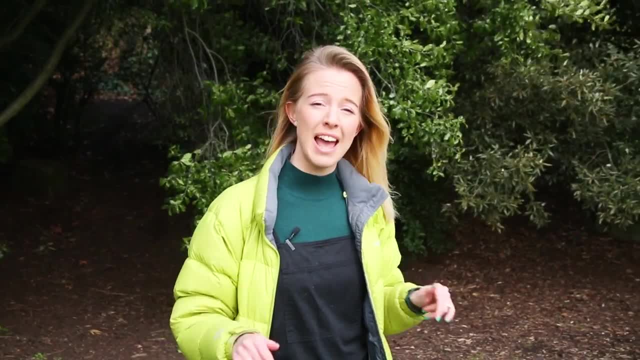 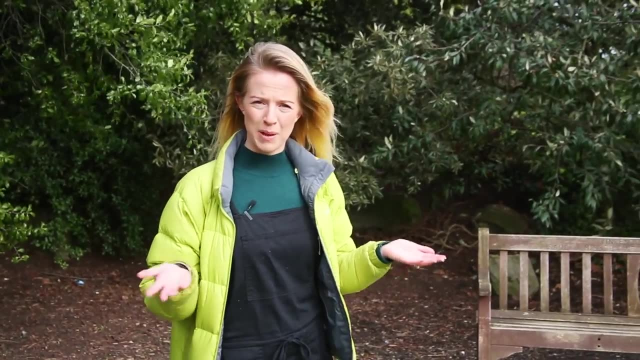 woods and the forests. 70% of land animals live in the woods and forests. If all of their habitats are cut down, then the animals will be gone. If the animals are gone, then they won't be able to play their part in the world. 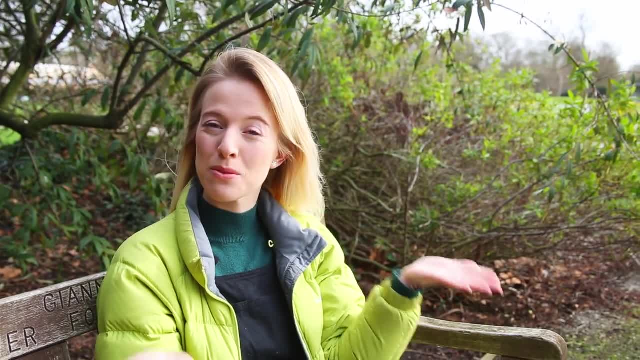 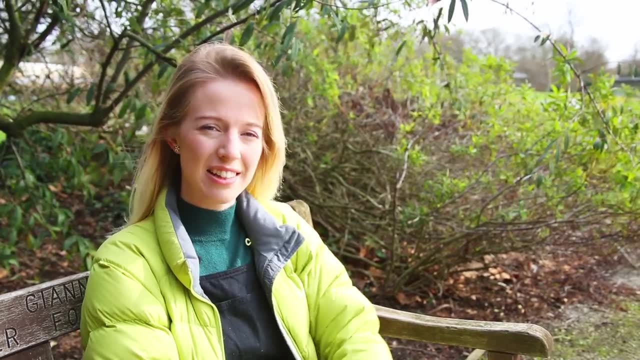 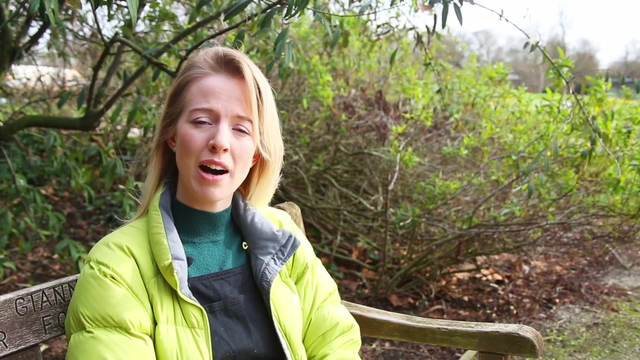 I'm about to go into the Battersea Children's Zoo to see some of the animals from different habitats around the world, But before I do that I need to answer some questions like: what is animal conservation? Animal conservation is taking care of wildlife and different animals. 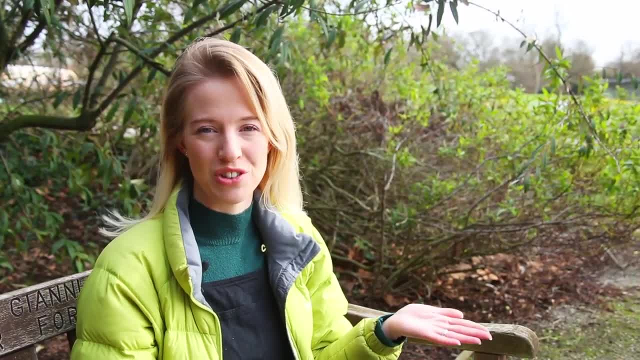 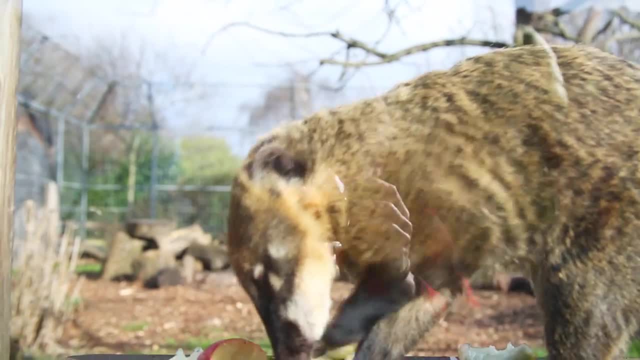 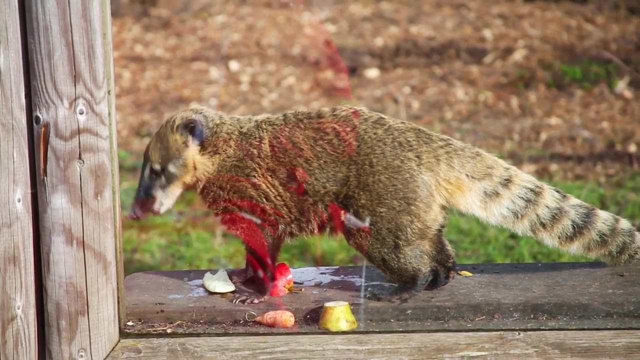 and their habitats, so they will always be around in the future. Why do these animals need protecting? Many of these animals need protecting because of the changes that are happening in their habitat or the environment, Whether it's directly or indirectly being done by humankind. some animals are finding it hard to survive and have or are going to. 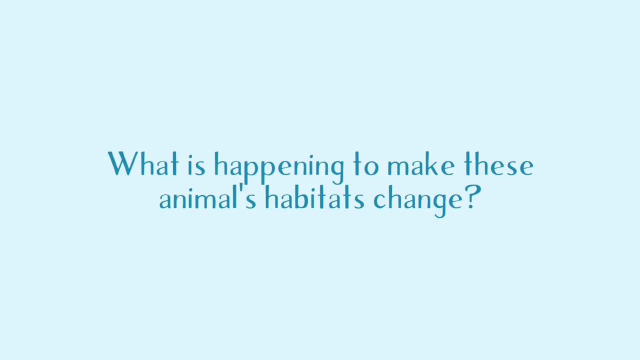 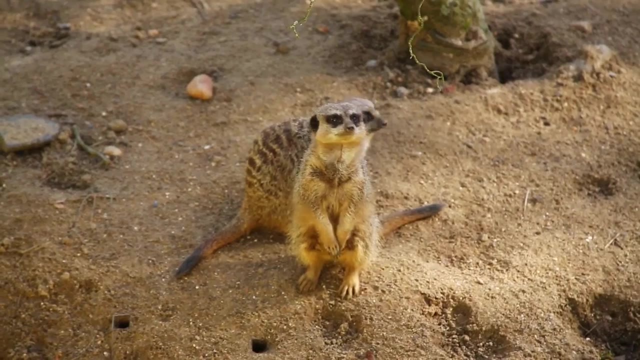 become extinct. What is happening to make these animals' habitats change? The human population is continuing to grow more and more. A side effect of this is that we need to use more and more of the earth's resources. The habitats are being affected by farming. 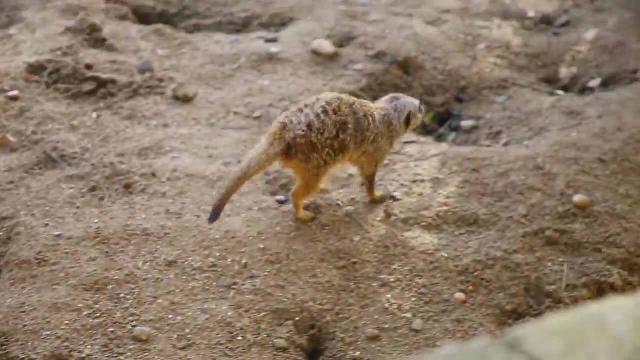 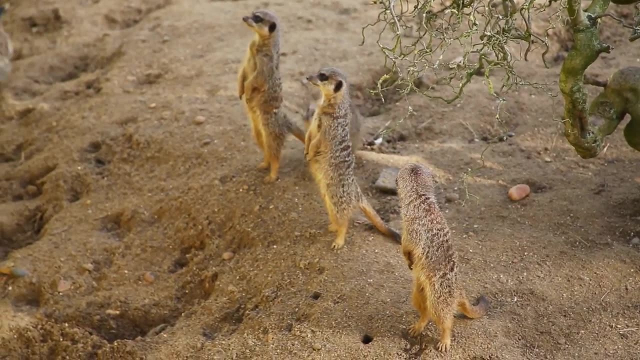 deforestation and overfishing. You may have also heard of climate change and global warming. This is where the earth is slowly heating up and making changes to the environment and then, in turn, making changes to the habitats. I don't think the polar bears would be very. 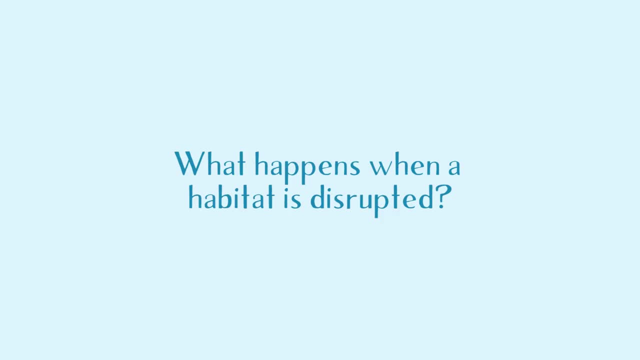 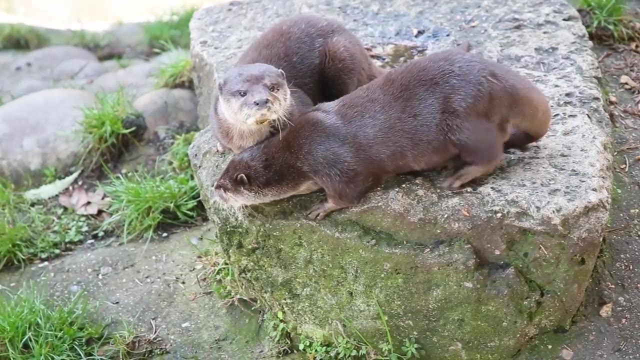 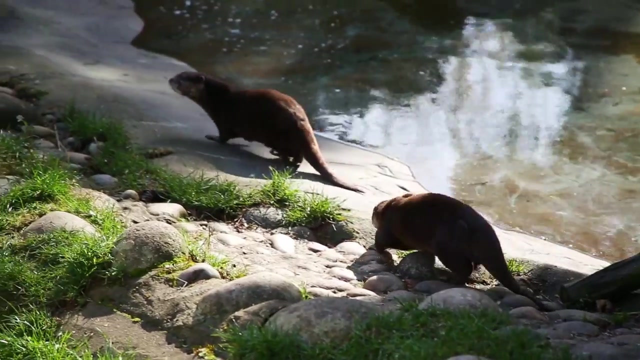 happy with a much warmer world. What happens when a habitat is disrupted? The world is a delicate place. Everything fits together like cogs in an enormous clock. When a habitat is disrupted, the animals that call it home don't deal with it very well. It then becomes: 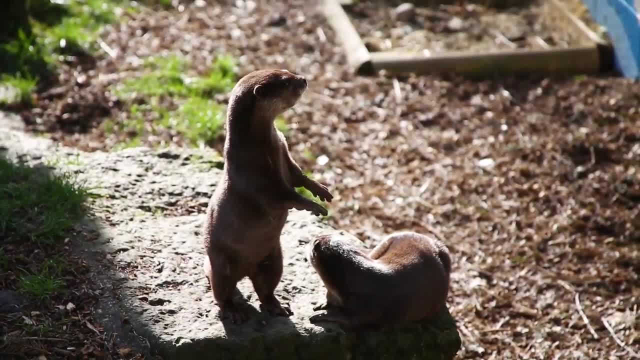 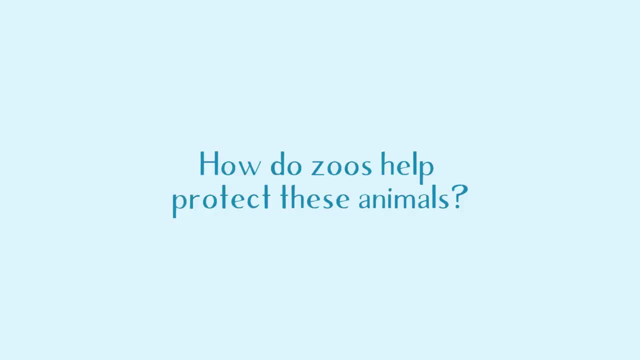 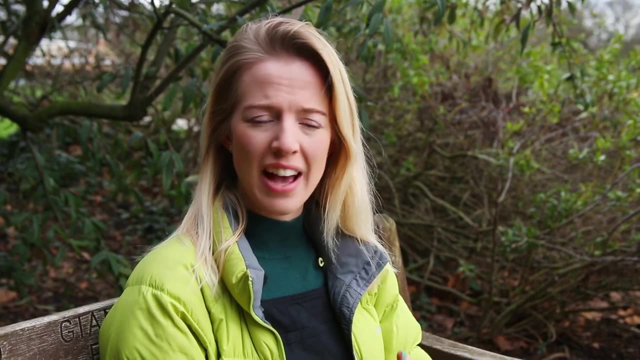 difficult to find food, shelter or even a mate, And that leads to there being a smaller population in that species of animal. How do zoos help protect these animals? Zoos and conservation centres play a very important role. Zoos provide a safe habitat for these. 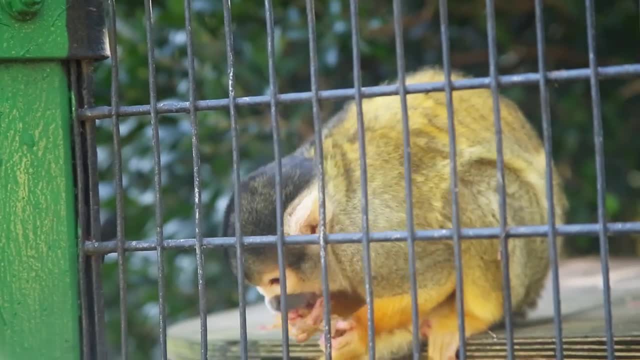 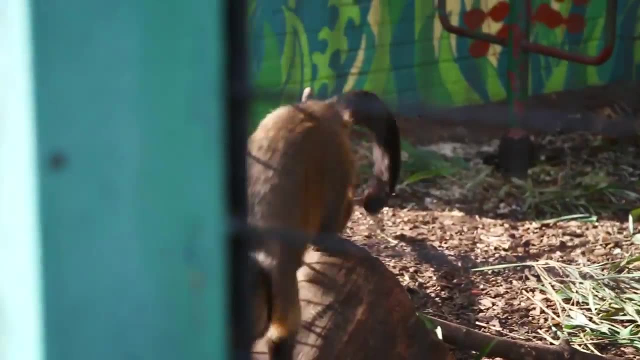 animals And conservationists are able to study, take care of and learn how to protect these animals. Lots of conservationists around the world are working on making sure they can reintroduce some of these animals back into the wild, For example, the South China.